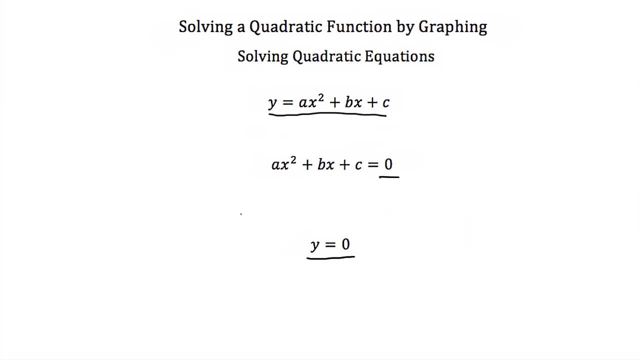 equal to zero. Well, if we were to graph this quadratic equation, we would be looking for places on that graph where y is equal to zero. Well, those are places where the graph crosses the x-axis. So we're looking for x-intercepts of this quadratic equation. Now, these x-intercepts. 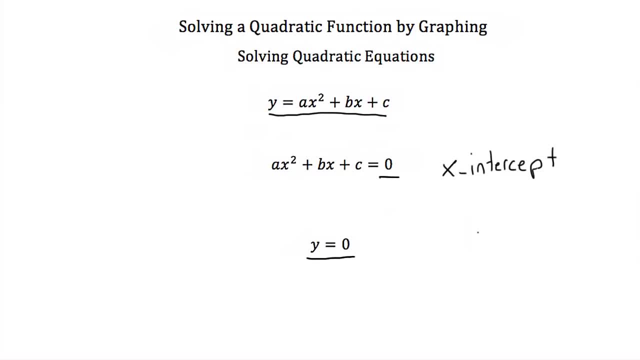 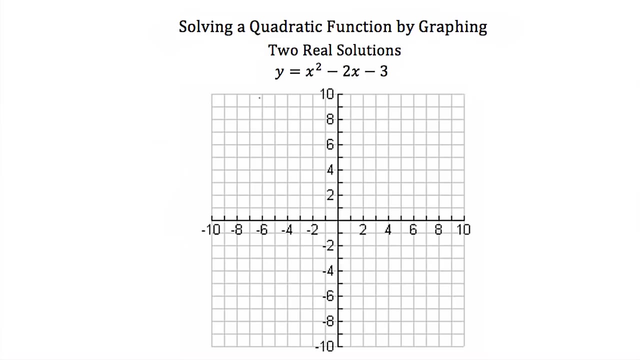 are sometimes called solutions, but they're also sometimes called zeros Or roots. Now, quadratic equations can have two solutions: one solution or zero solutions. Let's talk about the kind that have two real solutions. Here we have: y is equal to x squared minus 2x. 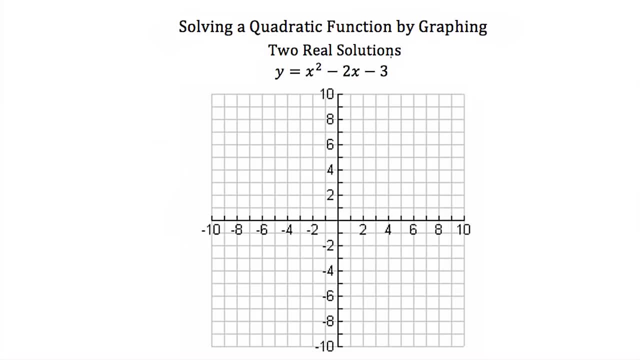 minus 3.. Now, if I wanted to find the zeros or the roots, or I wanted to solve this quadratic function, I could graph it. Now, if we graph it, the first step to graphing a quadratic is to find its axis of symmetry. So if we do that, we use the formula: x is equal to negative b over 2a. Now this: 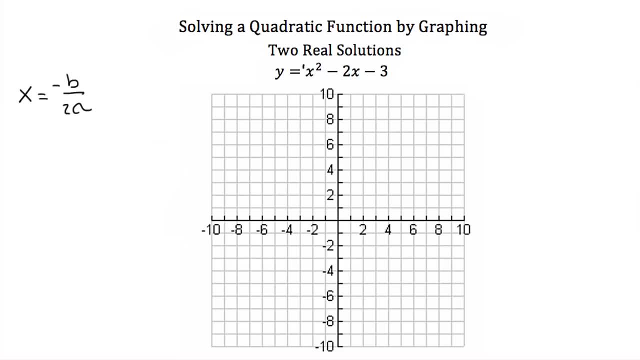 quadratic is already in standard form, which means my a is 1 and my b here is negative 2. So if I plug that in, I'll have a negative negative 2 over 2 times 1. This is equal to just 1, so our axis. 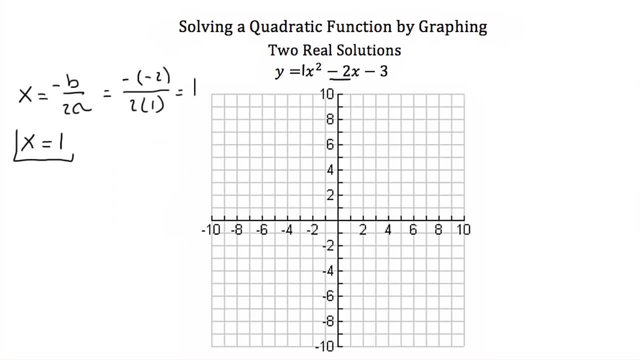 of symmetry then is: the line x is equal to 1.. Now that I have my axis of symmetry, my next step is to find my vertex, and I find that by plugging my x value of my axis of symmetry back into my original quadratic equation. If I do that, I'll have y is equal to 1 squared. 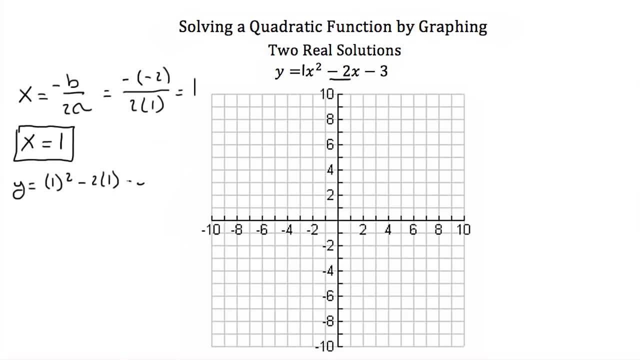 minus 2 times 1 minus 3.. Now 1 squared is 1 and minus 2 times 1 is minus 2, and then minus 3 again We have the y-coordinate of 1 minus 2 is negative. 1 minus 3 again would be negative 4. So 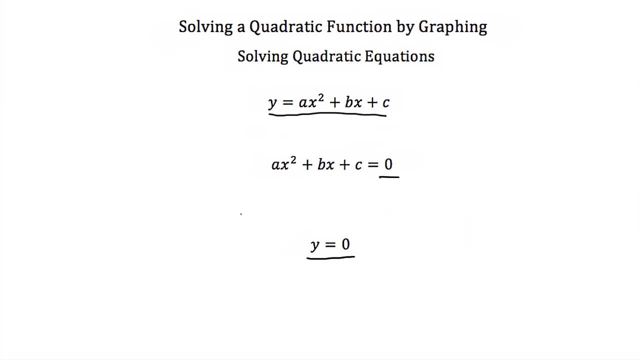 equal to zero. Well, if we were to graph this quadratic equation, we would be looking for places on that graph where y is equal to zero. Well, those are places where the graph crosses the x-axis. So we're looking for x-intercepts of this quadratic equation. Now, these x-intercepts. 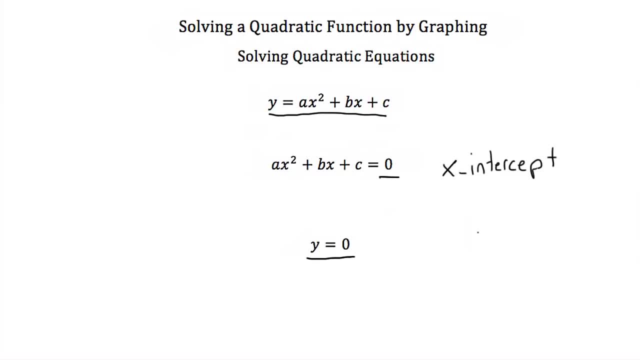 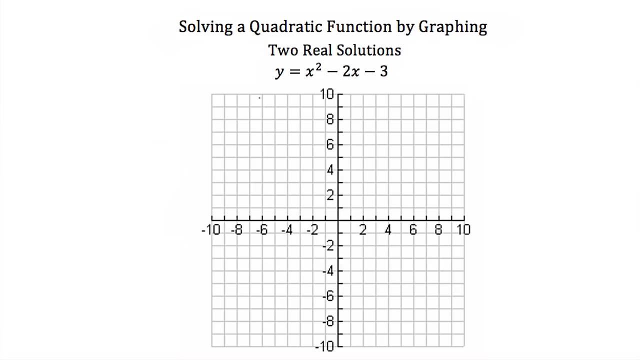 are sometimes called solutions, but they're also sometimes called zeros Or roots. Now, quadratic equations can have two solutions: one solution or zero solutions. Let's talk about the kind that have two real solutions. Here we have: y is equal to x squared. 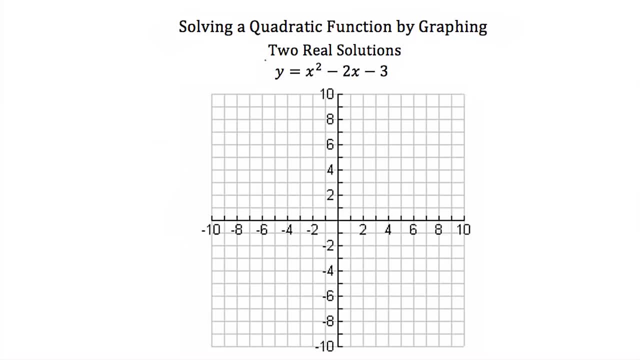 minus 2x minus 3.. Now, if I wanted to find the zeros or the roots, or I wanted to solve this quadratic function, I could graph it. Now, if we graph it, the first step to graphing a quadratic is to find its axis. 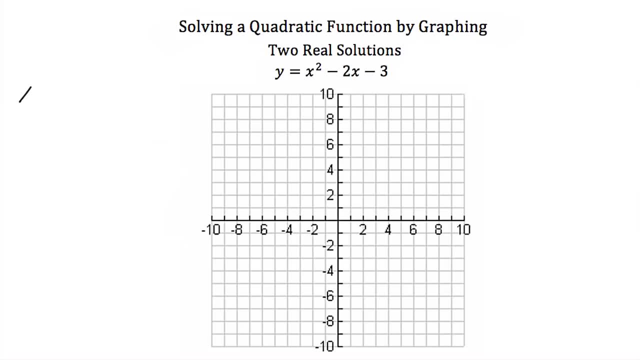 of symmetry. So if we do that we use the formula x is equal to negative b over 2a. Now this quadratic is already in standard form, which means my a is 1 and my b here is negative 2.. So if I 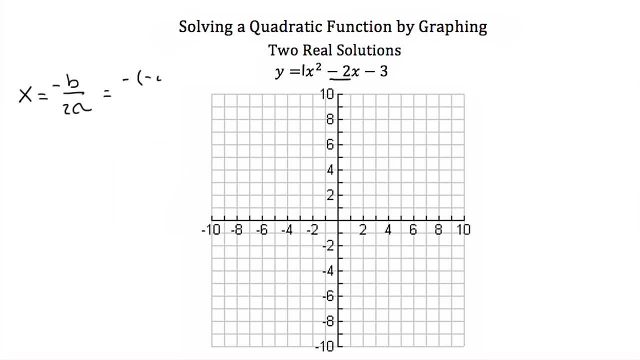 plug that in, I'll have a negative, negative 2 over 2 times 1.. This is equal to just 1, so our axis of symmetry then is: the line x is equal to 1.. Now that I have my axis of symmetry, my next step is: 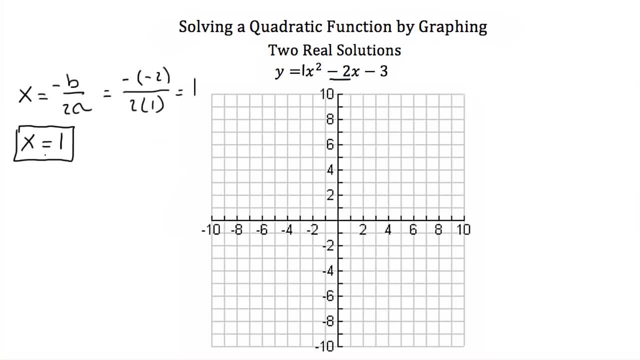 to find my vertex and I find that by plugging my x value of my axis of symmetry back into my original quadratic equation. If I do that, I'll have: y is equal to 1 squared minus 2 times 1 minus 3.. Now 1 squared is 1 and minus 2 times 1 is minus 2 and then minus 3. 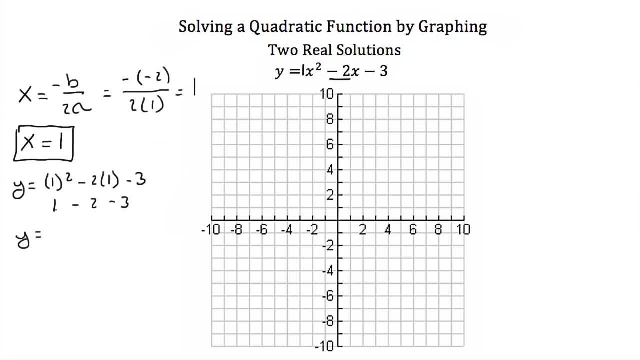 again We have the y-coordinate of 1 minus 2 is negative. 1 minus 3, again, would be negative 4.. So our vertex is the point 1, negative 4.. Now, lastly, we need one more point to graph this quadratic. I'm going to pick the y-intercept, because that's easy to solve for That. 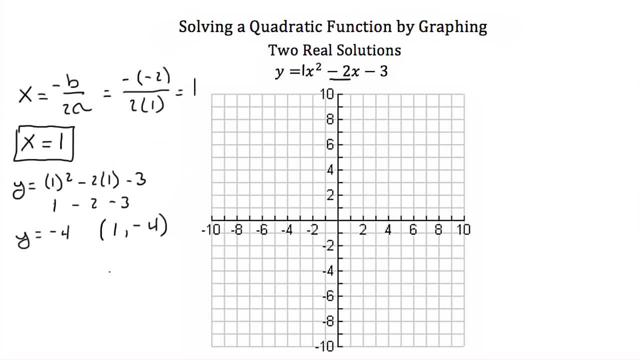 our vertex is the point 1, negative 4.. Now, lastly, we need one more point to graph this quadratic. I'm going to pick the y-intercept, because that's easy to solve, for That occurs when x is equal to 0. So if I plug that back into our quadratic, we'll have y is equal to. 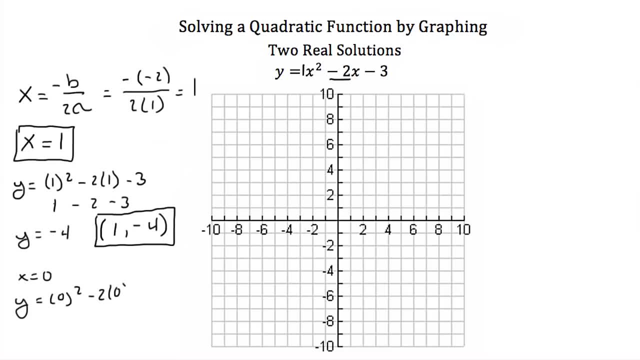 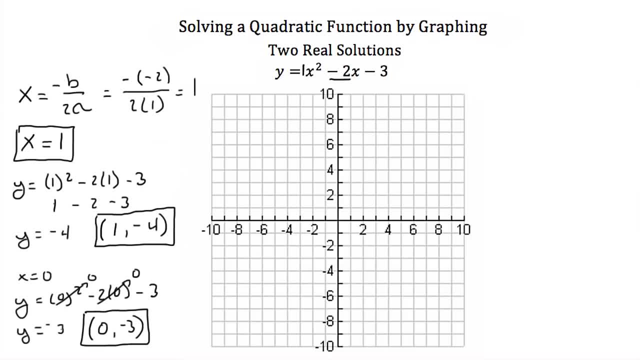 minus 3.. So let's plot all this. First we'll do our axis of symmetry. here It's the line x is equal to 1 and it'll look something like this: Next I'm going to plot my vertex, which is the point 1, negative 4, which 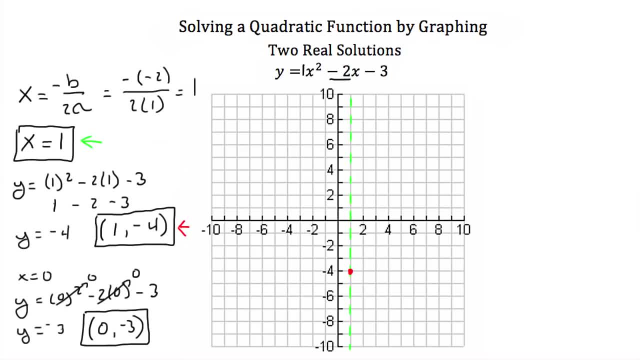 would be right here. And then I'm going to plot this other point that I found: 0, negative 3.. It's right here. Now, if I have a point one space to the left of my axis of symmetry, that means I also have a point one space to the. 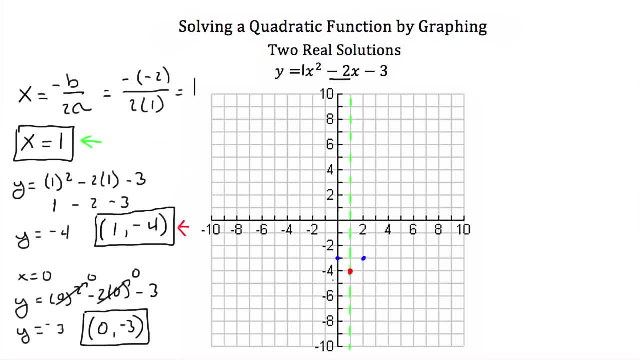 right of my axis of symmetry, So I'll have another point right there. Now I've got three points and I can connect the dots with a smooth curve And our graph will look something like that. Notice that we have two x-intercepts. We have one here at: x is equal to negative 1.. And 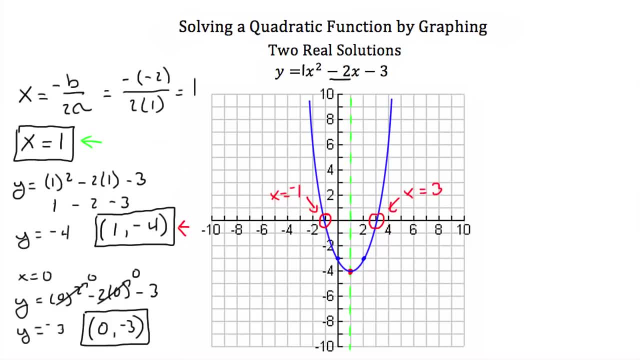 we have another one here, and x is equal to 3.. So the solutions or the roots or the zeros of this quadratic function here are: x is equal to negative 1 and x is equal to negative 3.. Now you can test these by just plugging them back in. 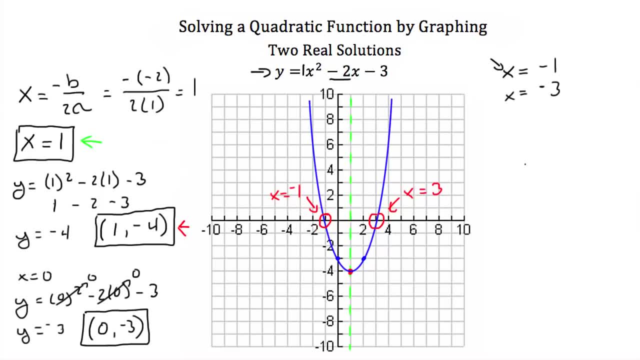 I'll test the first one here. x is equal to negative 1.. If we do that, we'll have: y is equal to negative 1 squared minus 2 times negative, 1 minus 3.. Now negative, 1 squared is 1.. Negative 2 times negative. 1 is a positive 2. 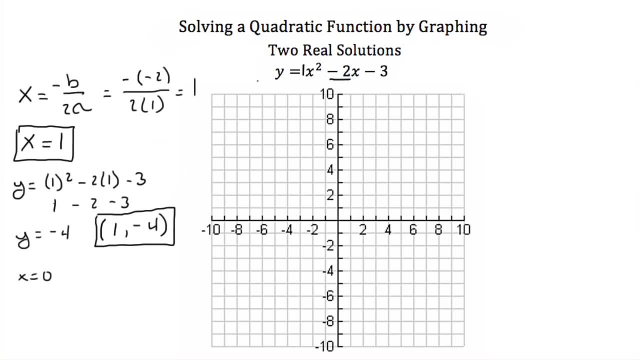 occurs when x is equal to 0. So if I plug that back into our quadratic, we'll have: y is equal to 0 squared minus 2 times 0 minus 3.. Now 0 squared is 0 and negative 2 times 0 is 0. So our y-coordinate 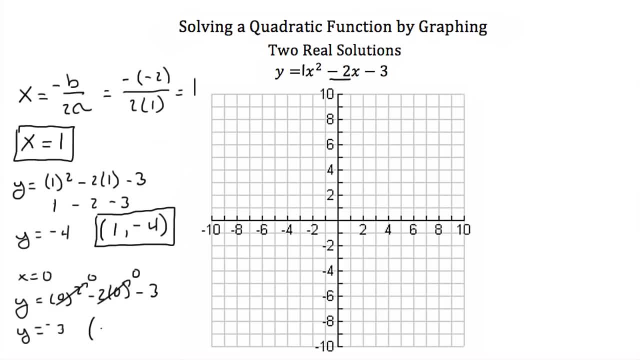 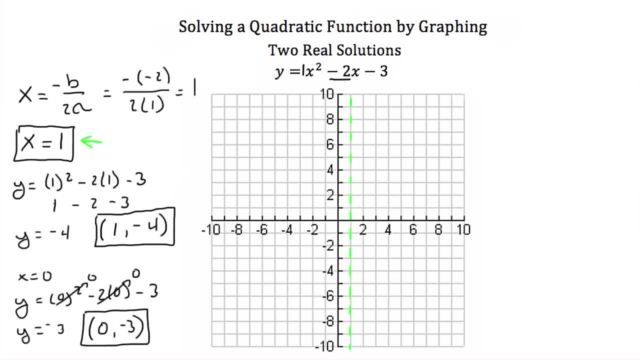 something like this: Next, I'm going to plot my vertex, which is the point 1, negative 4, which would be right here, And then I'm going to plot this other point that I found: 0, negative 3.. It's. 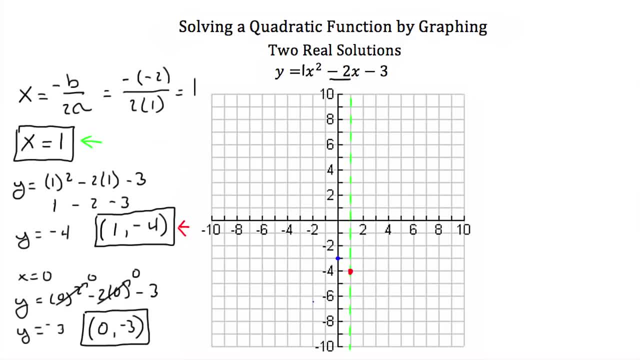 right here Now. if I have a point 1 spaced to the left of my axes of symmetry, that means I also have a point 1 spaced to the right of my axis of symmetry, So I'll have another point right there. Now I got three points and I can connect the dots with a. 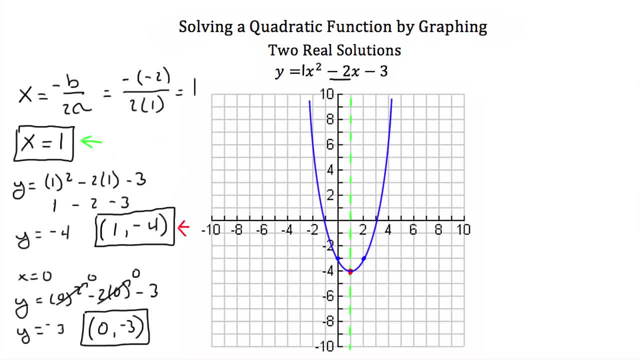 smooth curve And our graph will look something like that. Notice that we have two x intercepts. We have one here at X is equal to negative 1, and we have another one here, x is equal to 3.. So the solutions, or the roots, or the zeros of this quadratic. 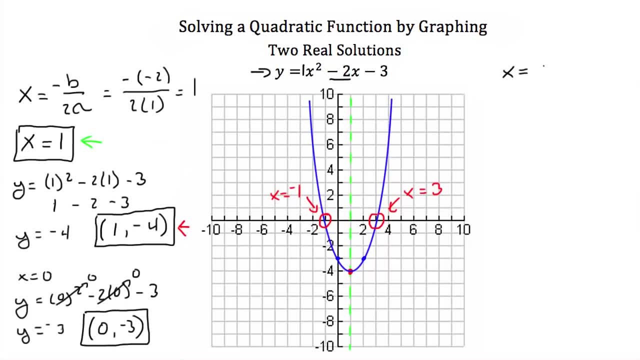 function. here are: x is equal to negative 1 and x is equal to negative 3.. Now you can test these by just plugging them back in. I'll test the first one here: x is equal to negative 1.. If we do that, we'll have: y is equal to negative 1. 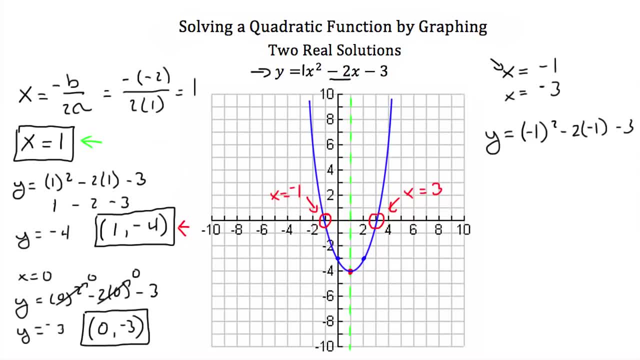 squared minus 2 times negative: 1 minus 3.. Now negative 1 squared is 1.. Negative 2 times negative: 1 is a positive 2 and then subtract 3.. 1 plus 2 is 3 minus 3 is. 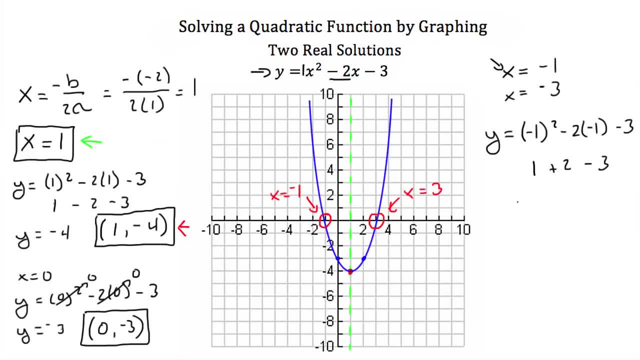 and then subtract 3.. 1 plus 2 is 3 minus 3 is y is equal to 0, which is what we were hoping would happen. So you can solve a quadratic function just by graphing it and looking at where it intercepts. 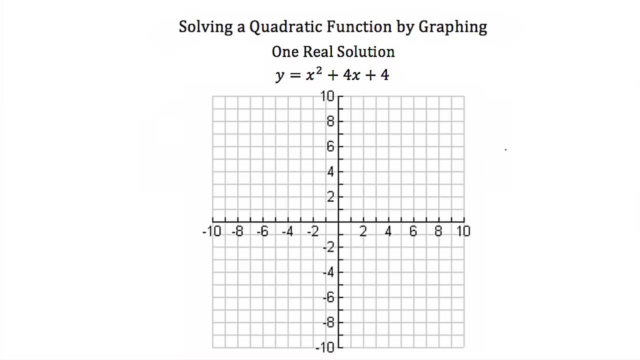 the x-axis. Now let's try solving a quadratic function that has only one real solution, or root, or 0.. Here we have: y is equal to x squared plus 4x plus 4.. Now we're going to follow the same steps. We're going to graph this. So first we're going to find its axis of symmetry. 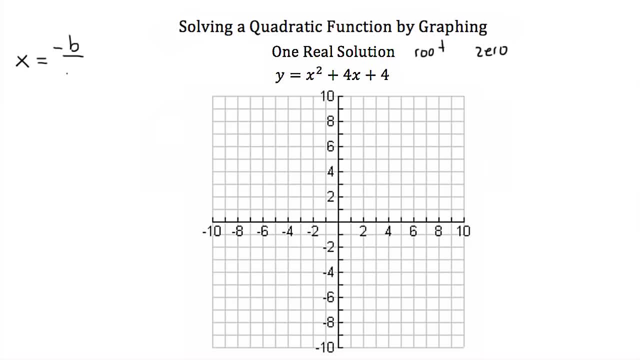 We're going to use the formula x is equal to negative b over 2a, where b is 4 and our a is 1.. Now if we plug that in, we'll have a negative 2x- 4 over 2 times 1. So a negative 4 over 2.. 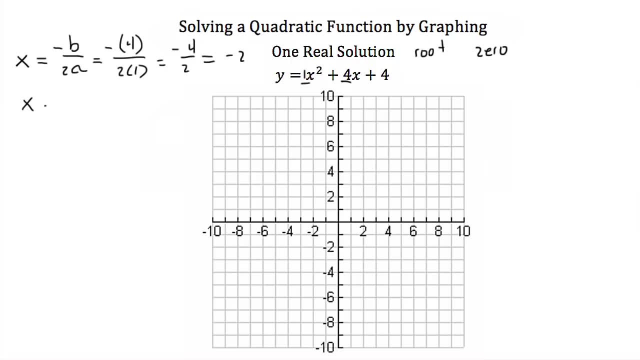 Or our axis of symmetry is: x is equal to negative 2.. Now that we've found our axis of symmetry, our vertex lies on that line, which means it has an x-coordinate of negative 2.. So we'll plug in negative 2 back into our quadratic to find the y-coordinate of our vertex. 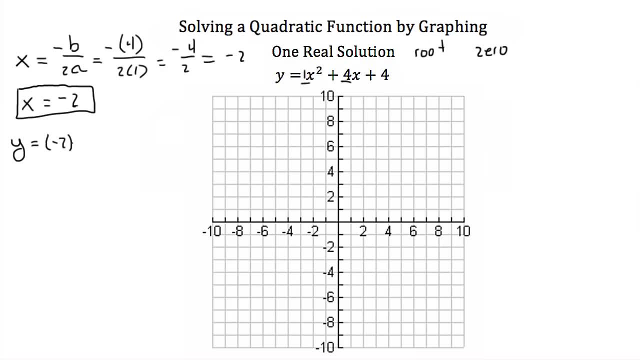 So we'll have: y is equal to negative 2 squared plus 4 times negative 2, plus 4x squared. Now negative 2 squared will be 4.. 4 times negative 2 is a negative 8, and then plus 4. 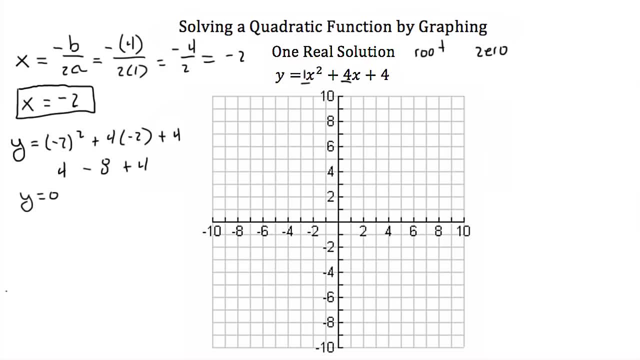 we get: y is equal to 0. So our vertex is the point negative 2, 0.. Now we're going to need one more point. I'm going to choose the y-intercept because it's easy to solve, for The y-intercept occurs when x is equal to 0. 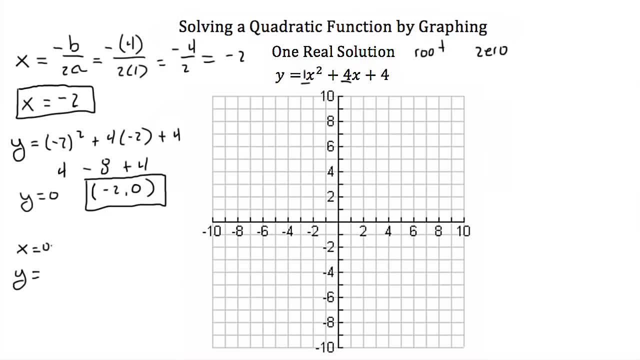 So if I plug that back into my equation, I'll have 0 squared plus 4 times 0 plus 4.. 0 squared is 0.. 4 times 0 is 0. So y is just equal to 4.. So our other point is going to be 0, 4.. 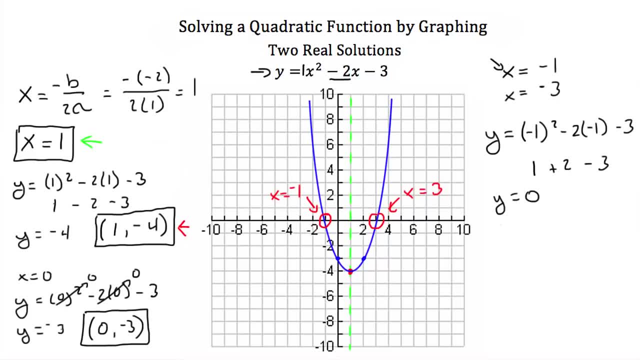 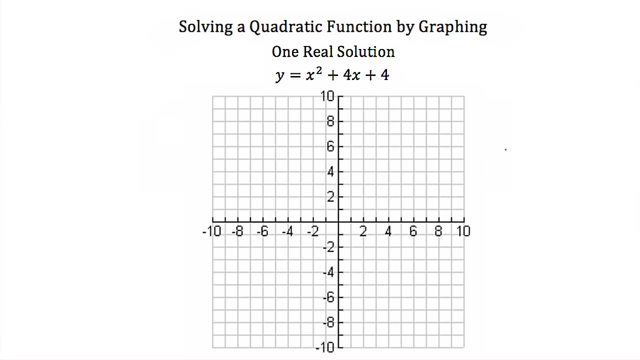 y is equal to 0, which is what we were hoping would happen. So you can solve a quadratic function just by graphing it and looking at where it intercepts the x axis. Now let's try solving a quadratic function that has only one real solution, or root, or 0.. Here 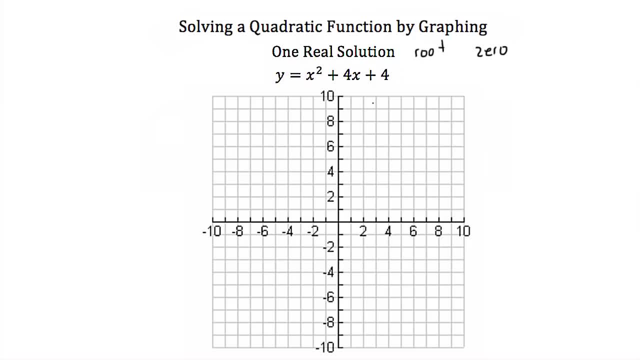 we have, y is equal to x squared plus 4x plus 4.. Now we're going to follow the same steps. We're going to graph this. So first we're going to find its axis, asymmetry. We're going to use the formula: x is equal to negative b over 2a, where b is: 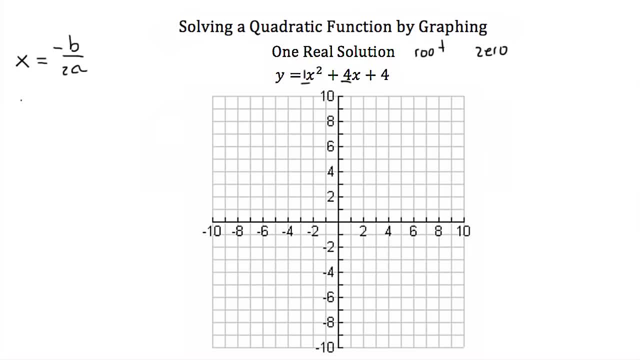 4 and our a is 1.. Now if we plug that in, we'll have a negative 4 over 2 times 1.. So a negative 4 over 2, or our axis of symmetry is x, is equal to negative 2.. Now that we found our axis of symmetry, our vertex lies on: 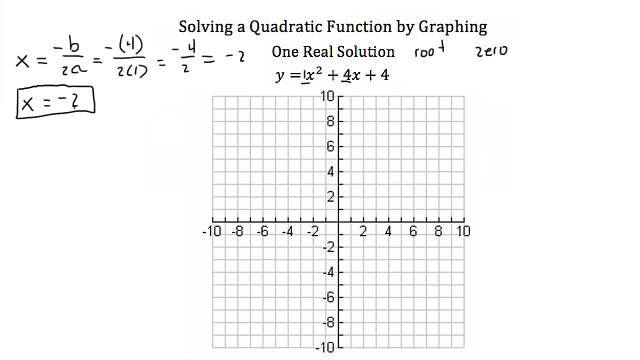 that line, which means it has an x coordinate of negative 2.. So we'll plug in negative 2 back into our quadratic to find the y coordinate of our vertex. So we'll have: y is equal to negative 2 squared plus 4 times negative 2. 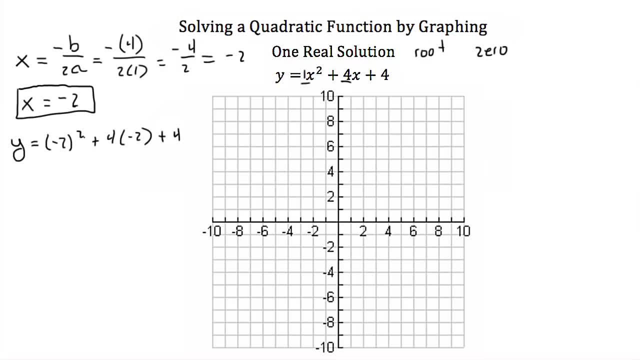 plus 4.. Now negative 2 squared will be 4.. 4 times negative 2 is a negative 8, and then plus 4 we get y is equal to 0. So our vertex is the point negative 2, 0.. Now 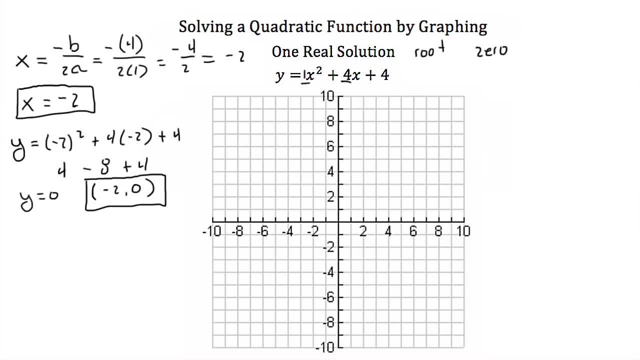 we're going to need one more point. I'm going to choose the y-intercept because it's easy to solve, for The y-intercept occurs when x is equal to 0. So if I plug that back into my equation, I'll have 0 squared plus 4 times 0 plus 4.. 0 squared is 0.. 4 times 0 is 0.. 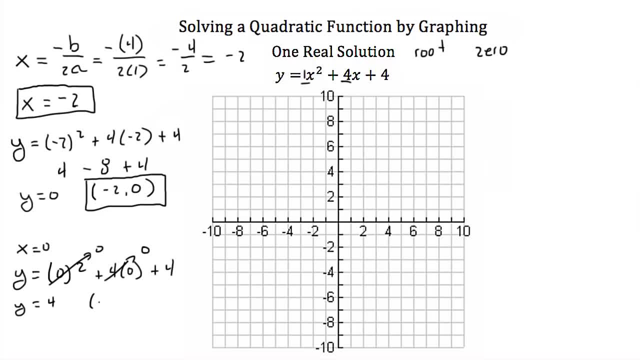 So y is just equal to 4.. So our other point is going to be 0, 4.. So let's plot this stuff. Here we have our axis of symmetry at x is equal to negative 2, and it's going to look something like this: Next we'll plot our vertex, which is the. 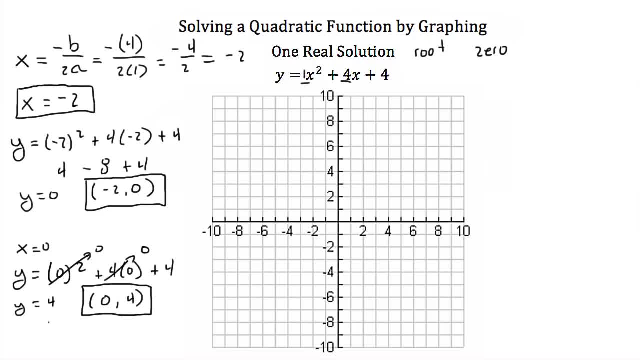 So let's plot this stuff. Here we have our axis of symmetry at x is equal to negative 2.. And it's going to look something like this: Next we'll plot our vertex, which is the point: negative 2, 0, which is right here. 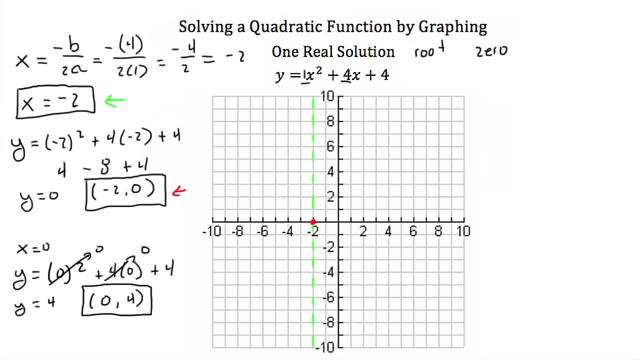 And then I'm going to plot my y-intercept, which is at 0, 4, which is up here. Now, if I have a point 2 spaces to the right of my axis of symmetry, then this parabola has a point 2 spaces to the right of my axis of symmetry. 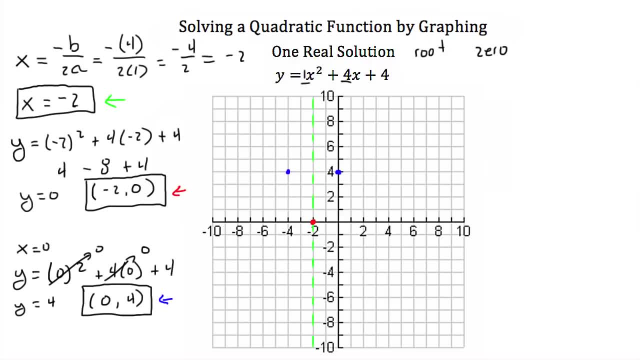 Then this parabola has a point: 2 spaces to the right of my axis of symmetry. Then this parabola has a point 2 spaces to the right of my axis of symmetry. So I have my three points and I connect them with a smooth curve. 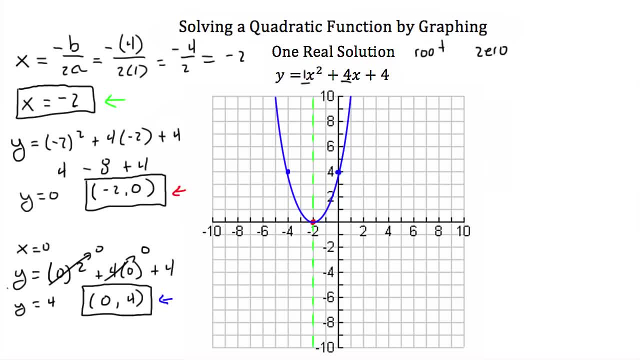 So there's the graph of x squared plus 4x plus 4.. Notice that I have only one x-intercept. It's my vertex. So, since I only have one x-intercept, I have only one real solution. This is the point. 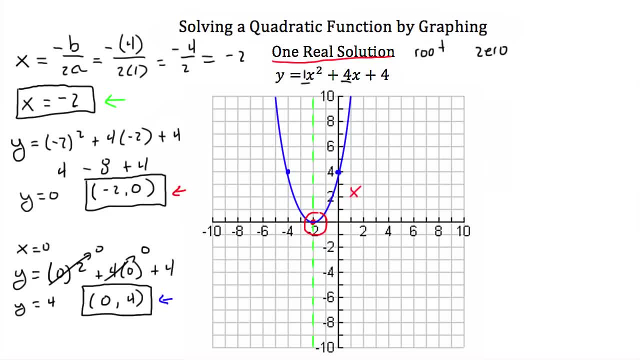 That's a negative 2: 0.. Or my solution is: x is equal to negative 2.. Now we can test this: If we plug in x is equal to negative 2 into our quadratic, We should get y is equal to zero. 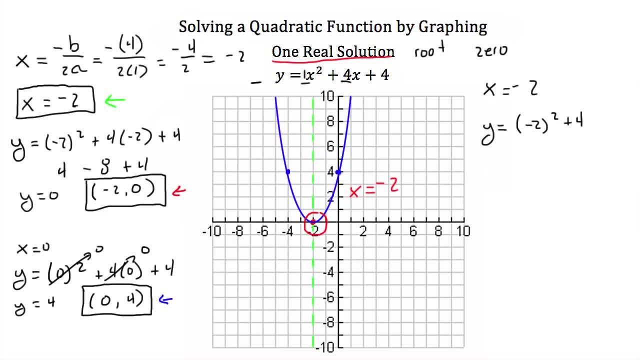 We'll have negative 2 squared plus 4 times negative, 2 plus 4.. Negative 2 squared is 4.. 4 times negative 2 is a negative 8, and then plus 4.. 4 minus 8 is negative, 4 plus 4.. 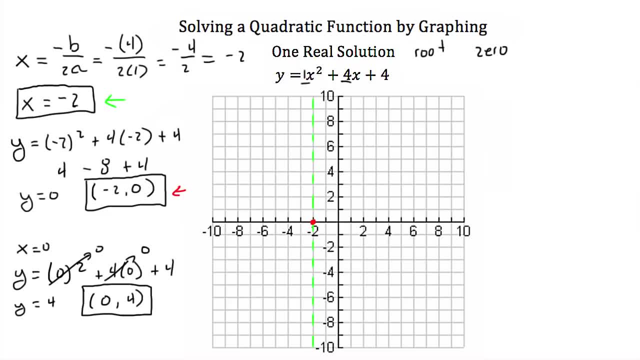 point negative 2, 0, which is right here. And then I'm going to plot my y-intercept, which is at 0, 4, which is up here. Now, if I have a point 2 spaces to the right of my axis of symmetry, 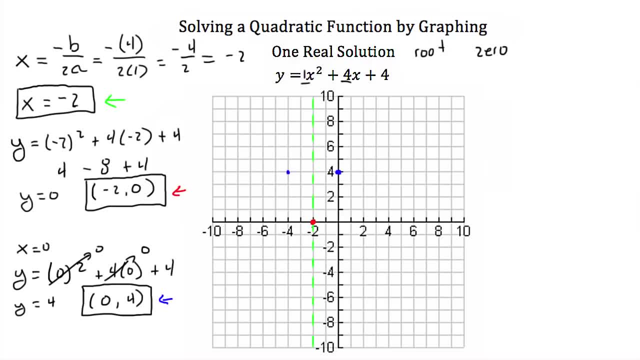 then this 연� will equal to 0.4, which is 0.. хорош And congratulations You. mouth-mouse was awesome. Thanks a bunch. Have a wet and心going day. Bye, Bye, bye. the left of my x is a symmetry, So I have my three points and I connect them with. 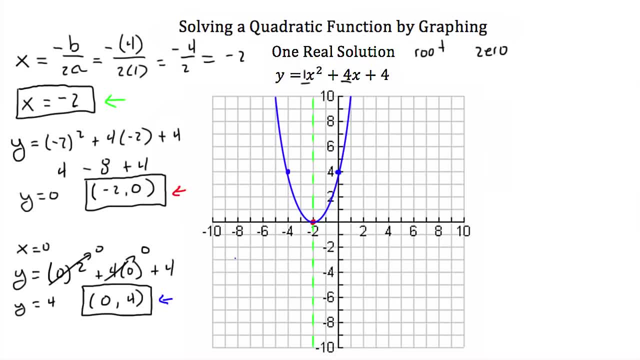 a smooth curve. So there's the graph of x squared plus 4x plus 4.. Notice that I have only one x-intercept. It's my vertex. So since I only have one x-intercept, I have only one real solution. This is the point: negative 2, 0.. Or my solution is: x is equal. 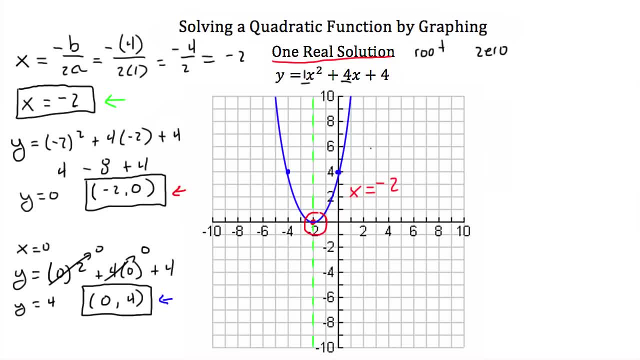 to negative 2.. Now we can test this: If we plug in x is equal to negative 2 into our quadratic, we should get y is equal to 0. So we'll have negative 2 squared plus 4 times negative 2 plus 4.. Negative 2 squared is 4.. 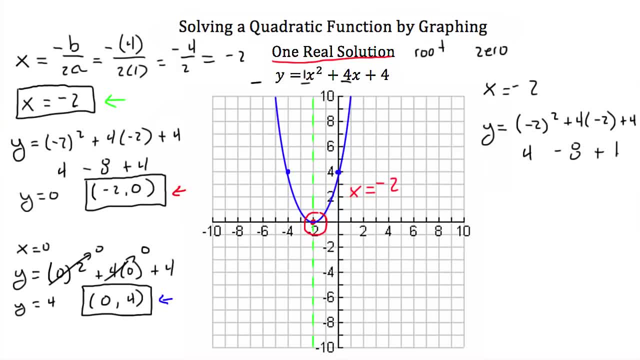 4 times negative. 2 is a negative 8, and then plus 4.. 4 minus 8 is negative. 4 plus 4 is indeed 0.. So our solution then of y is equal to x squared plus 4x plus 4 is x is equal. 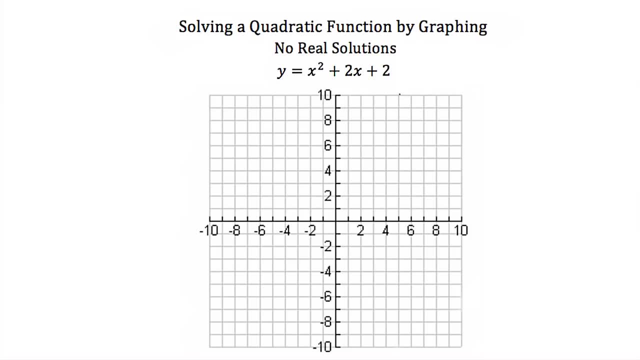 to negative 2.. So now we're going to talk about our last type of quadratic, One that has no real solutions. Here we have: y is equal to x squared plus 2x plus 2.. Now again, if we wanted to solve this by graphing, we would first plot the quadratic function. 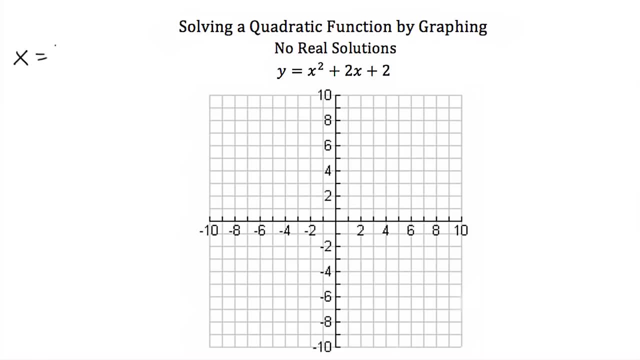 So the first thing we do is find our axis of symmetry. using the formula x is equal to negative b over 2a. Our b is 2.. Our a is 1.. So we'll have negative 2 over 2 times 1.. 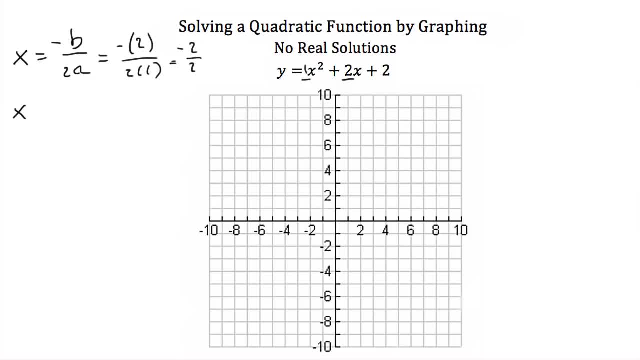 Negative 2 over 2.. So our axis of symmetry is: x is equal to negative 2 squared plus 4x, plus 4x Negative 1.. Now I need to find my vertex, So I plug in my axis of symmetry coordinate. 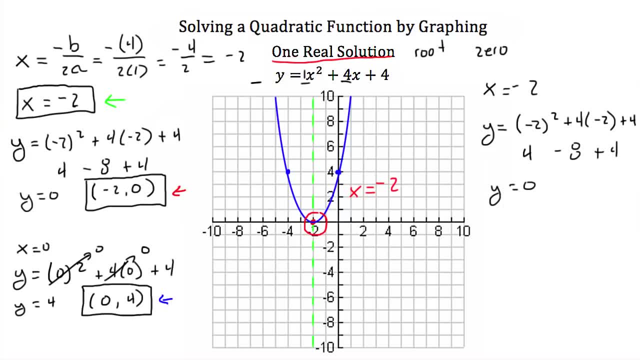 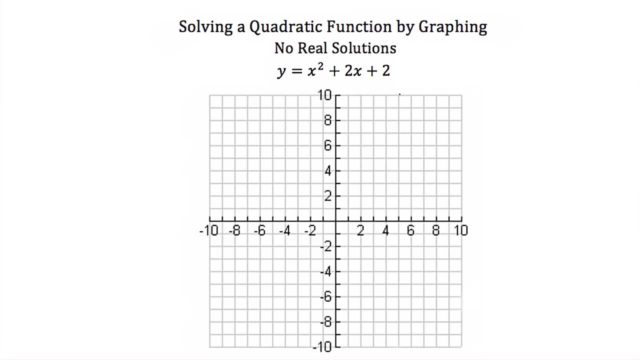 is indeed 0.. So our solution then of y is equal to x squared plus 4x plus 4 is x is equal to negative 2.. So now we're going to talk about our last type of quadratic, one that has no real 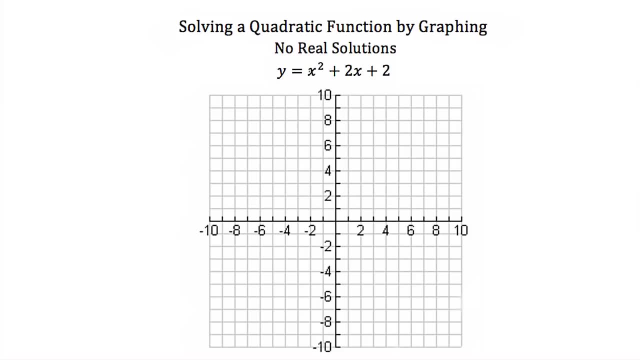 solutions Here we have: y is equal to x squared plus 2x plus 2.. Now again, if we wanted to solve this by graphing, we would first plot the quadratic function. So the first thing we do is find our axis of symmetry using the formula: x is equal to negative b over 2a. Our b is 2, our a is. 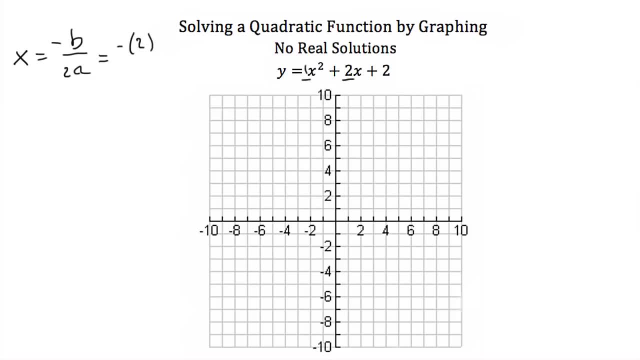 1.. So we'll have negative 2 over 2 times 1, negative 2 over 2.. So our axis of symmetry is: x is equal to negative 1.. Now I need to find my vertex, So I plug in my axis of symmetry coordinate back into my original equation. 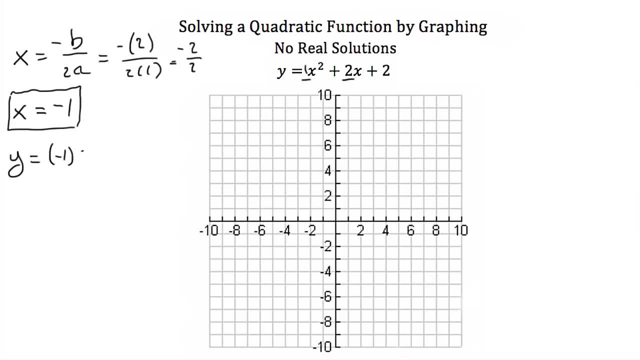 We'll have: y is equal to negative 1 squared plus 2 times negative, 1 plus 2.. Negative 1 squared is 1.. 2 times negative, 1 is negative, 2 and then plus 2.. My y coordinate then is 1, or my vertex is the point. 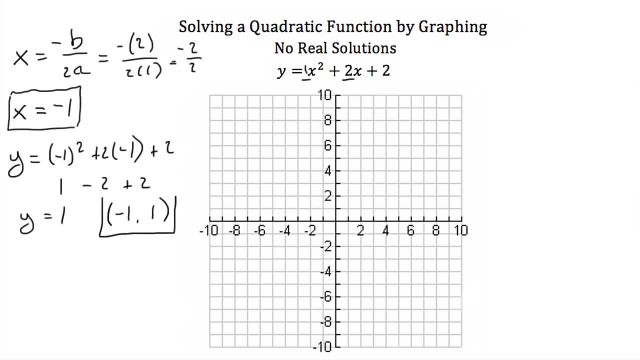 negative: 1, 1.. Now I'm going to need one other point. So again I'm going to try the y intercept, or when x is equal to 0. So I'll plug that in: of y is equal to 0 squared plus 2 times 0 plus 2.. 0 squared is 0.. 2 times 0 is 0.. 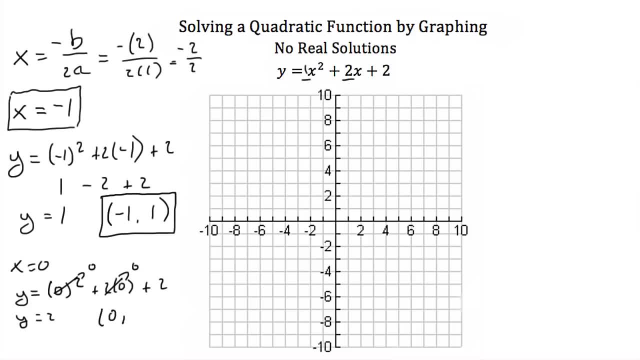 So y is equal to 2.. So we have the point 0, 2.. So I'm going to plot all this. First, I'm going to plot my axis of symmetry. The line x is equal to negative 1, it's going to look something like this: 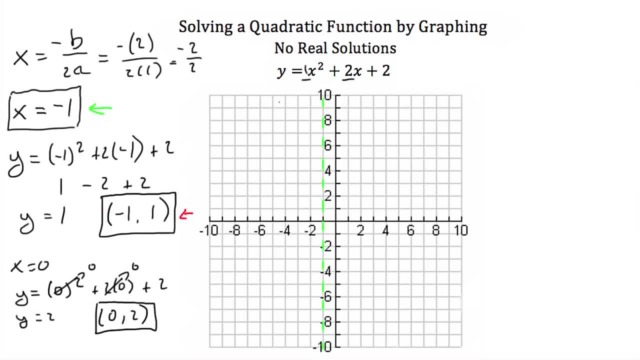 Next, I'm going to plot my vertex- It's the point negative, 1, 1,, which is right there. And then I'm going to plot my y intercept here at 0, 2,, which is right here. Now, if I have a point one space to the right of my axis of symmetry, this is a parabola. 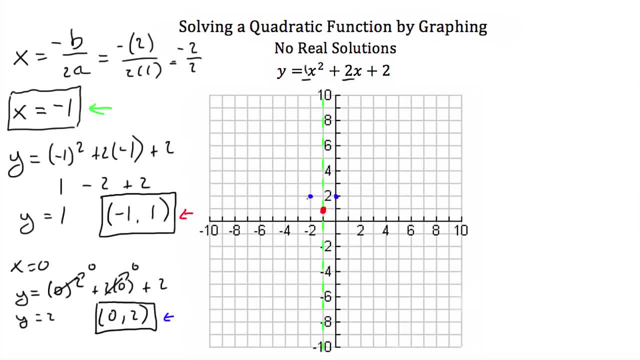 So I also have a space 1 to the left, left of my axis of symmetry. Connect these with a smooth curve which will look something like that. Here's the graph of x squared plus 2x plus 2.. Notice that it does not cross the x-axis. so there are no x-intercepts. there are no. 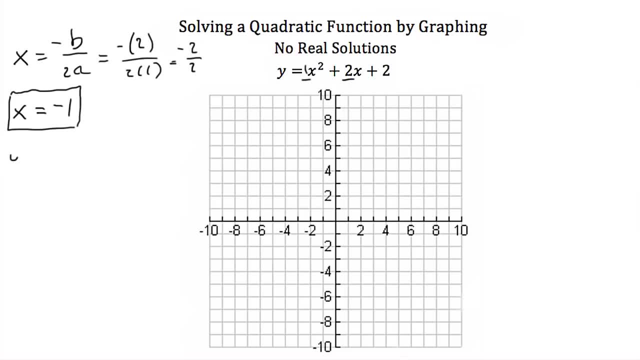 back into my original equation, We'll have: y is equal to negative 1 squared plus 2 times negative, 1 plus 2.. Negative 1 squared is 1.. 2 times negative, 1 is negative, 2 and then plus 2.. 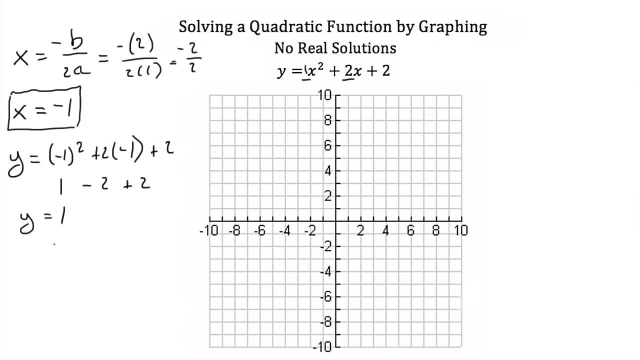 My y coordinate then is 1.. For my vertex is the point negative 1, 1.. Now I'm going to need one other point. So again I'm going to try the y intercept, or when x is equal to 0. So I'll plug that in. 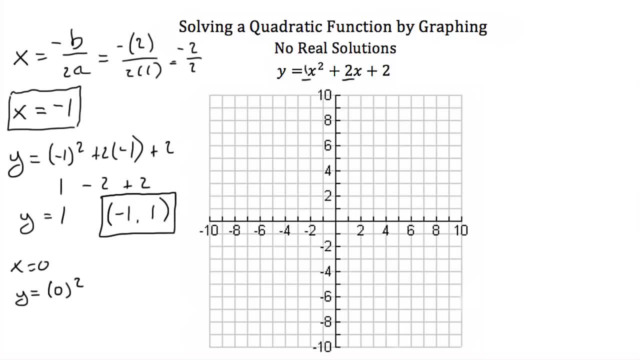 Y is equal to 0 squared plus 2 times 0 plus 2.. 0 squared is 0.. 2 times 0 is 0, So y is equal to 2.. So we have the point. So I'm going to plot all this. First I'm going to plot my axis of symmetry. 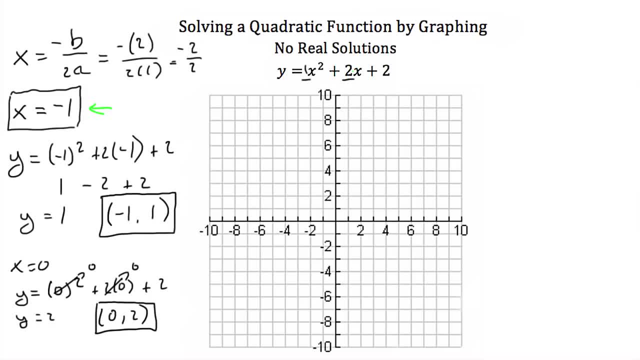 It's, the line x is equal to negative 1, and it's going to look something like this. Next I'm going to plot my vertex- It's the point negative 1, 1,, which is right there. And then I'm going to plot my y-intercept here at 0, 2,, which is right here. 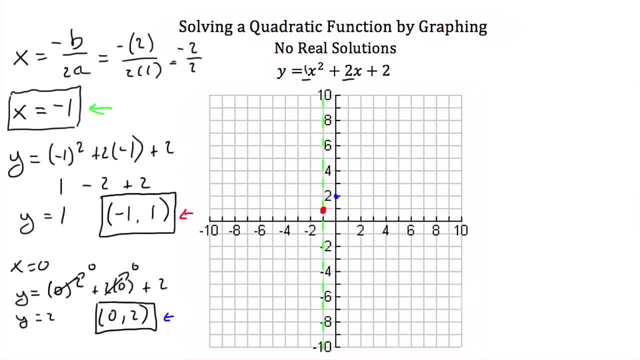 Now, if I have a point, one space to the right of my axis of symmetry- this is a parabola- So I also have a space 1 to the left of my axis of symmetry. Connect these with a smooth curve which will look something like that: 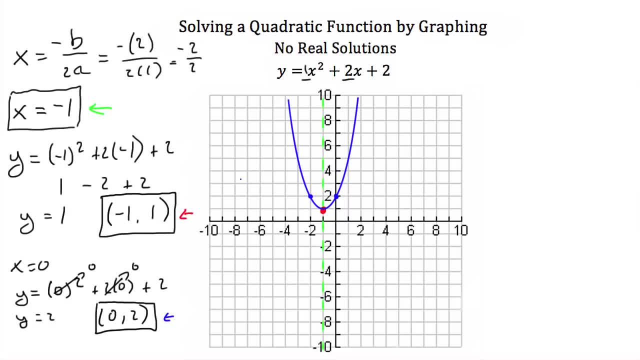 Here's the graph of x squared plus 2x plus 2.. Notice that it does not cross the x-axis. So there are no x-intercepts, There are no zeros, There are no roots, So this one has no real solutions. 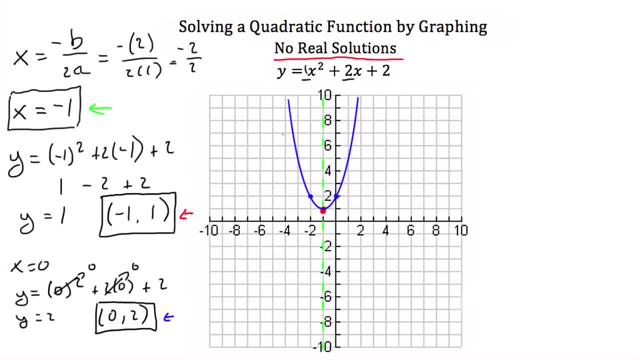 We can tell that just from the graph. So we've graphed quadratics with two real solutions, one real solution and now no real solutions. So that completes the tutorial on solving a quadratic function by graphing.